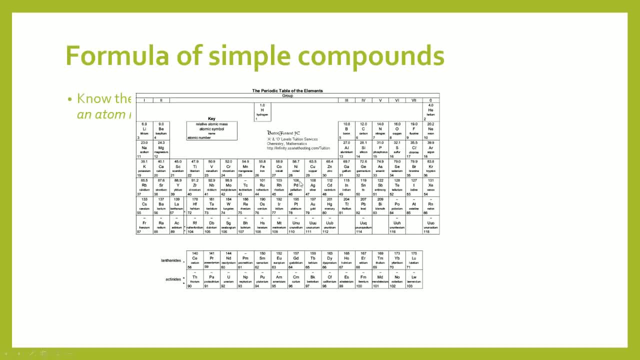 2. It skips the middle here, which is transition meals you don't really need to know, and then it goes to group 3,, 4,, 5,, 6, and 7. We'll learn about the periodic table in a bit more. 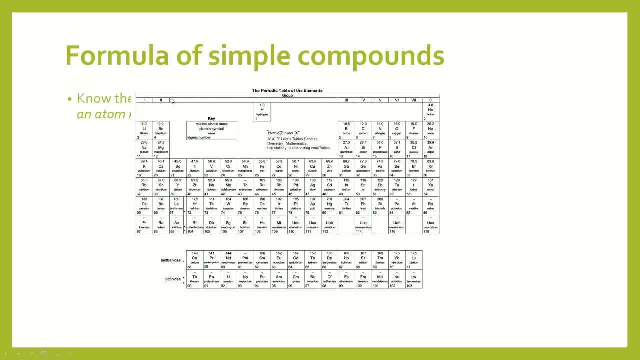 detail later, but these columns or groups are really important because it tells you how many electrons these atoms within the group have in their outer shell. So beryllium, for example, is in group 2, therefore it has 2 electrons in its outer shell, whereas nitrogen 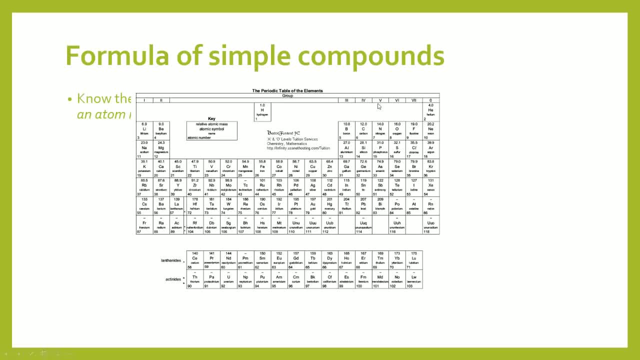 has 5.. Why that's important is because, if you looked at my previous video, it means that you can determine what an atom needs to gain a full outer shell. So if you look at my previous video, it means that you can determine what an atom needs to gain a full 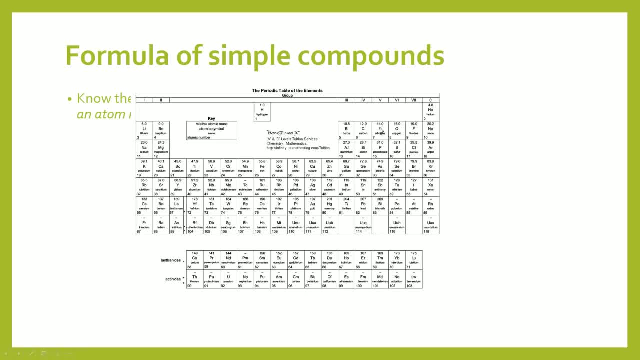 shell. So this wants to put in 2 electrons. So we can really start by explaining what an atom needs to do in order to gain a full outer shell. For example, in terms of nitrogen, it needs to gain 3 electrons, because it has 5. So it just needs 3 more to achieve a full. 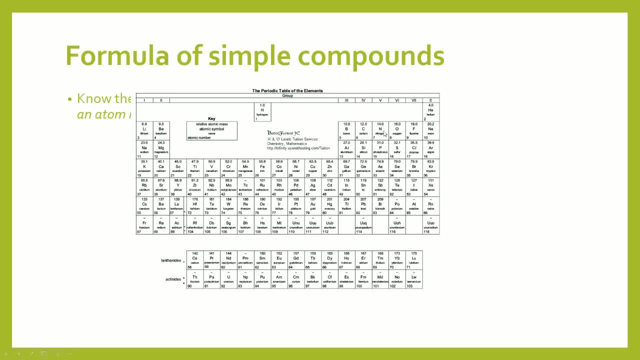 outer shell, which is a lot easier than losing 5 electrons. So non-metals on the right side of the periodic table will tend to gain electrons to fulfil their atomic stability, Whereas on the left hand side, for example, lithium ets got one electron and it's outer shell. 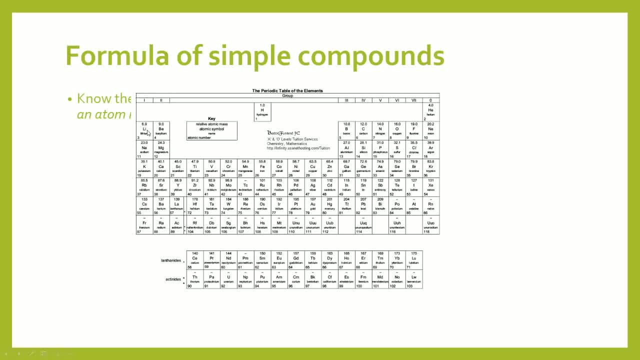 so it'd rather lose one electron to make itself have a full outer shell. And the valency is important because it also gives you the charge of whatever you're looking at, of the ion, of the atom, For example lithium here, if it turns from an atom to an ion. 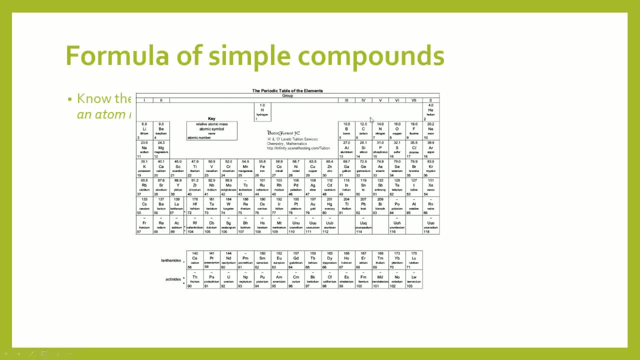 well, it's going to be losing one electron, so the charge is going to be minus one. For oxygen, for example, it's in group six, so it needs two extra electrons. When it gains those two electrons, then it's going to have a charge of minus two. 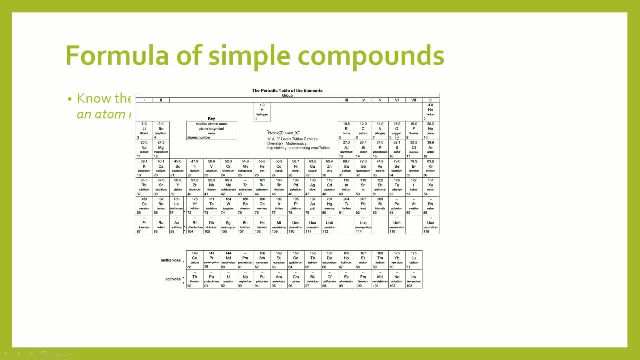 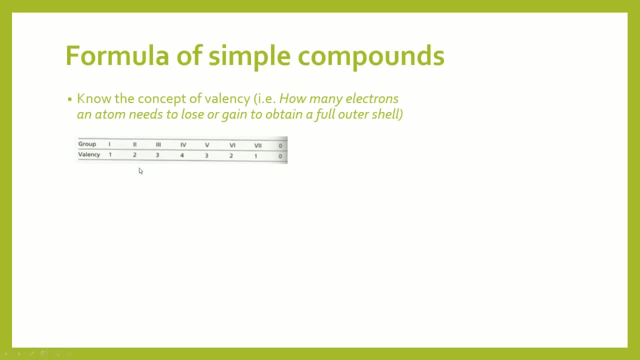 This will become a bit more easier for you as you progress through the course, But anyway, what you need to understand is mainly the concept of valency, right? So group one valency of one, because it needs to lose one electron. 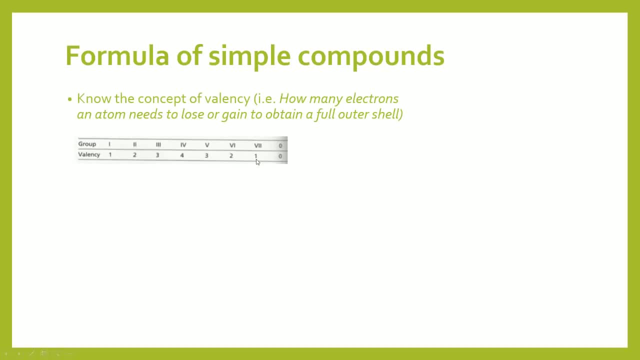 Group seven: valency of one also because it needs to gain one electron. So, whether it's losing or gaining, the valency is how many electrons need to be gained or lost in order to achieve a full outer shell, and that's very, very important. 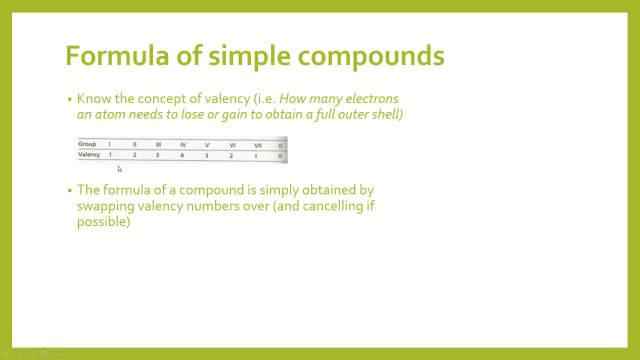 So the formula of a compound is simply. it's basically obtained by swapping the valency numbers over- okay, and cancelling if possible. For example, you have potassium oxide and you've got the valency of one for potassium and two for oxygen. 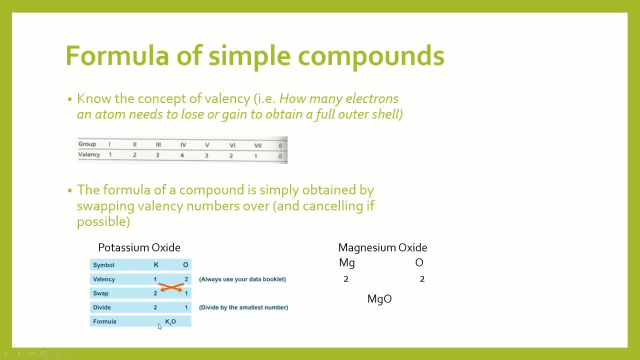 You swap the numbers and what you get is K2O, that is the formula for potassium oxide, Magnesium oxide. you have valency of two for magnesium, and also oxygen has a valency of two. You swap the numbers over, but in this case you can cancel it out. and if you can cancel, you must cancel. 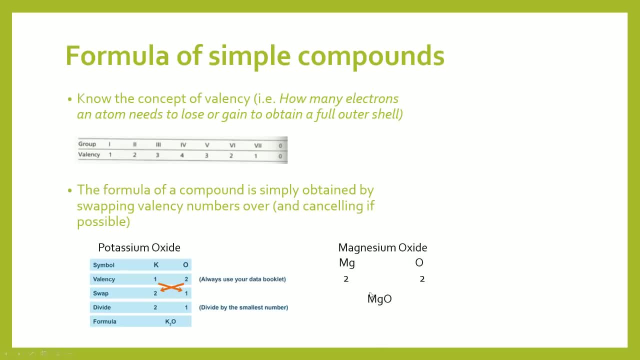 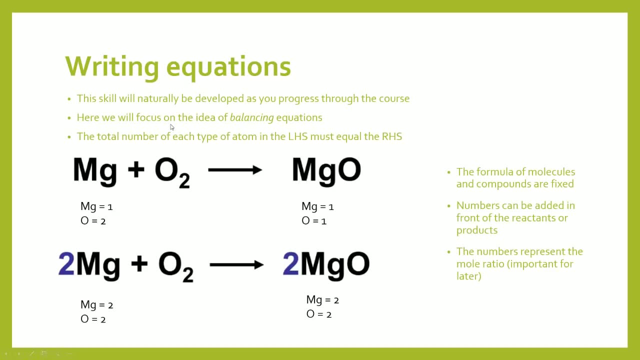 What that leaves is MgO. so that's fairly simple. So the second step is to be able to write simple equations right. This skill will actually naturally be developed as you sort of progress through the course. as you learn. you know certain rules of different chemicals reacting with different other substances and things like that. 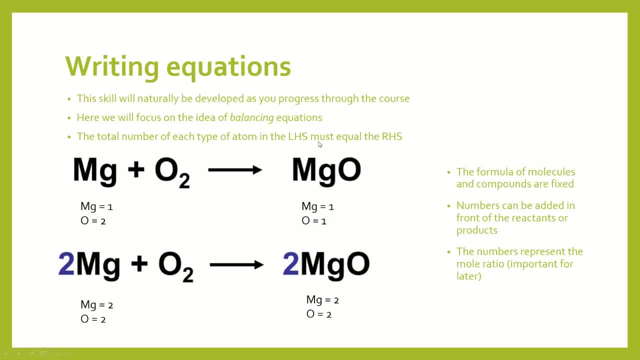 but here we'll focus on the idea of balancing equations, because this is crucial. So the total number of each type of atom in the left-hand side of the equation has to equal the right-hand side. You can't just- atoms can't disappear or be gained from one side to the other. 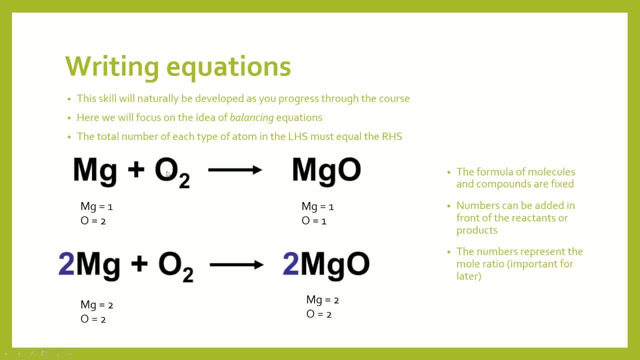 It has to be absolutely equal. As you can see, magnesium plus oxygen giving you magnesium oxide. in this example, you can see that the equation is not balanced, Whereas you've got two octian on the left-hand side but only one oxygen on the right. 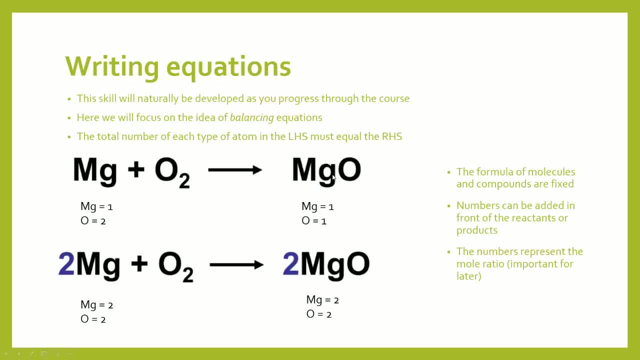 So what can you do to fix this? Well, you can't change the formula itself. You know that magnesium oxide has the formula of MgO. You can't simply just make it MgO2 to try to balance the equation. but, for example, why would we believe that if the ratio is so high? 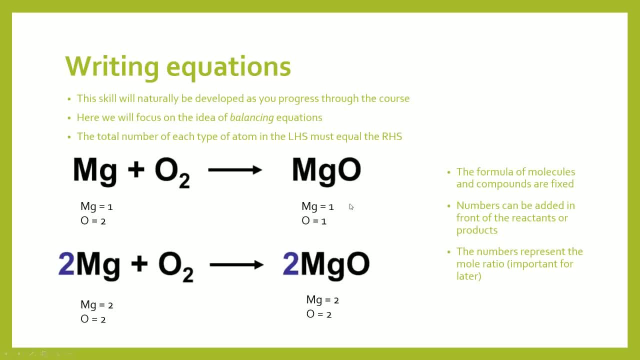 equation, just to add an extra option here, that you cannot do that. so? but what you can do is add numbers to the front of the compound or whatever it is, and so, for example, in this case, you can add a two in front of magnesium oxide, giving you two magnesium on the right hand side of the equation. so therefore you have to. 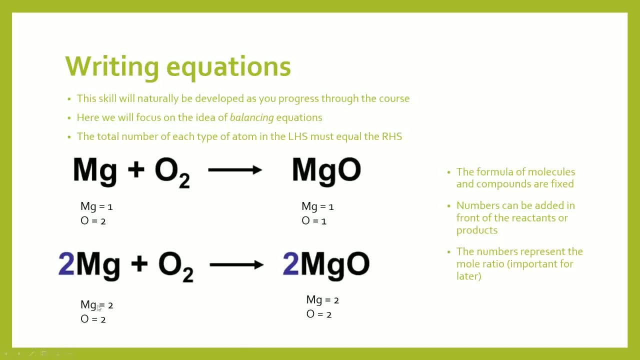 add two onto the left hand side and we, when you do this, you have a balanced chemical equation whereby you have, you know, an equal number of atoms of each particular element on both sides of the equation, and so these big numbers that you put in front actually represent the mole ratio. so every magnesium atom that 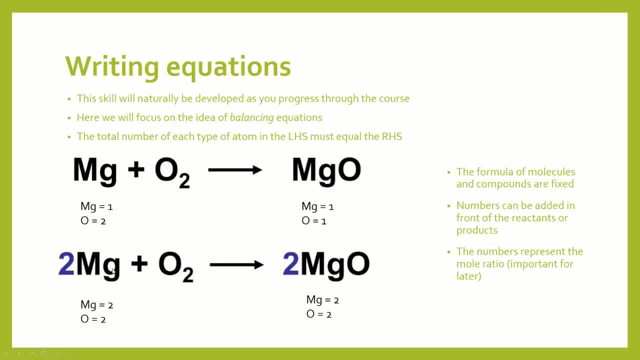 is used in the equation, I suppose, or in the reaction, because it has a two in front and oxygen theoretically only has a one in front because it's got nothing there. it tells you that for every magnesium, because it's a two to one ratio, for every magnesium that is used, only half of oxygen is used, and we'll learn more. 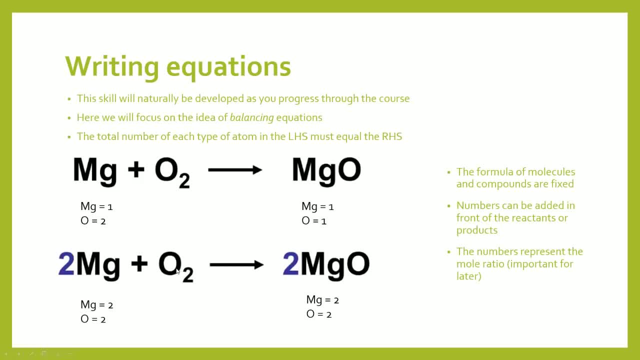 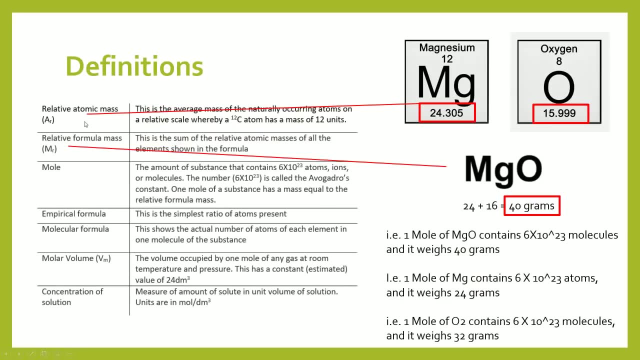 about the mole ratios later, and this becomes really important when you're doing calculations for stoichiometry. so there's a couple of definitions that you need to get your head around. we've got the relative atomic, atomic sorry mass that's represented as the AR, and this is the average mass of the naturally 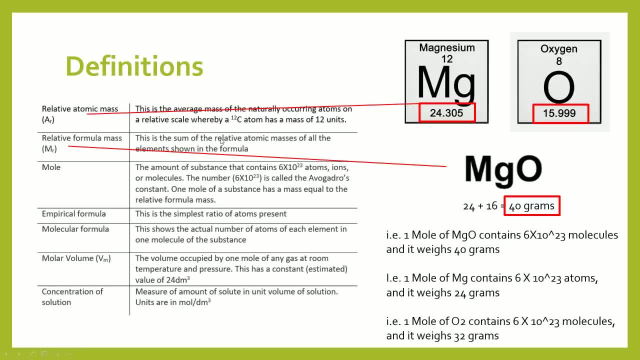 occurring atoms on a relative scale, whereby the carbon has a mass of 12 units, you don't need to know anything about how it distrib agriculture, but you just need to use the weighted number. so, whatever the Advanced numbers, of atoms have specific mass numbers, and if it is negative, then we 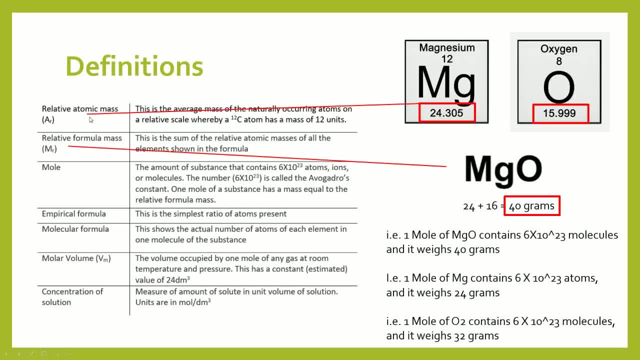 Um overall, if you look at The Periodic Table, how much Number table of atoms? Okay, so the definition itself is not really important, but what you do need to know here as that if you look at the periodic table, you've got the mass number. you should be familiar with mass number, proton number we're talking about. 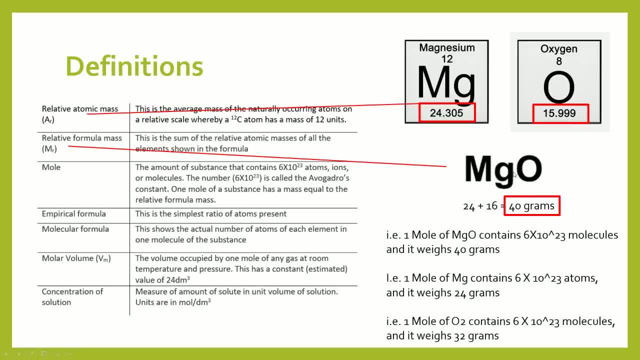 of all the different relative atomic masses inside the compound. in this case you've got magnesium, which is, you know, an ar of 24, and oxygen, which has an ar of 16. so the relative formula mass of magnesium oxide is just the sum of all those, which is basically 24 plus 16, giving 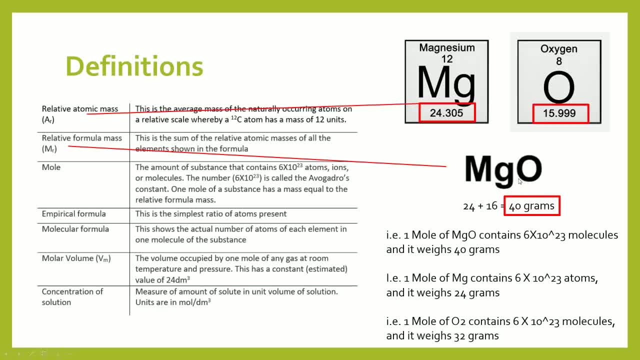 you 40 grams. okay, now, this is all relative, it's relative mass, but it's important, and so magnesium oxide here has 40 grams. and why this is important is because one mole- okay, so one mole- of any substance is. this is basically defined as the amount of substance that contains six to the 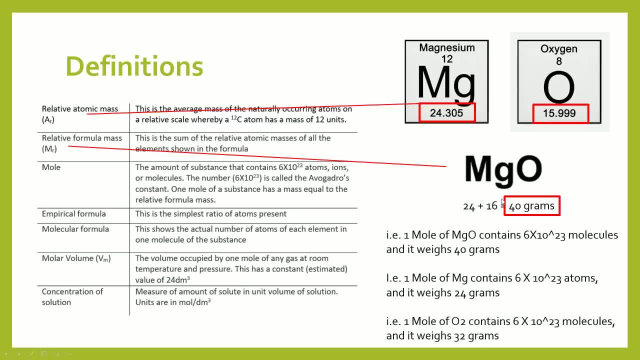 power six times 10 to the power of 23 atoms, ions or molecules within that substance. okay, and that specific number is called the avogadro's constant. what's really important here, of course, is the idea that one mole of any particular substance will have the weight of the relative formula mass of that. 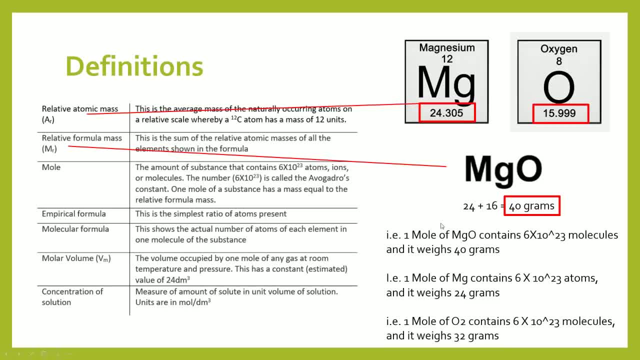 compound, okay. so, for example, when we take a look at magnesium oxide, here one mole of MDO- okay- is defined as you know, the amount of substances that contain six times 10 to the power of 23 magnesium oxide molecules, and all together that one mole will weigh. 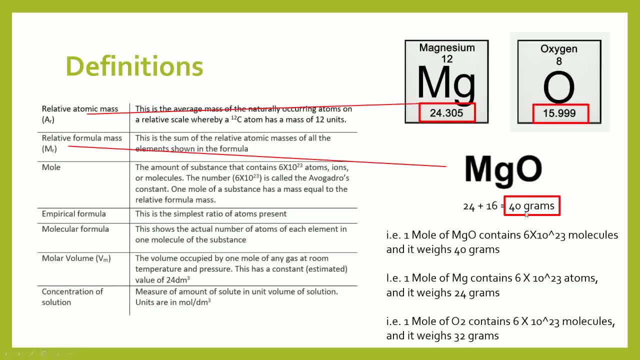 40 grams and, as you can see, 40 grams is the relative formula mass. okay, One mole of magnesium will contain six times, six times four times is six times 10, to the power of 23 magnesium atoms. it will weigh 24 grams. okay, which is just the. 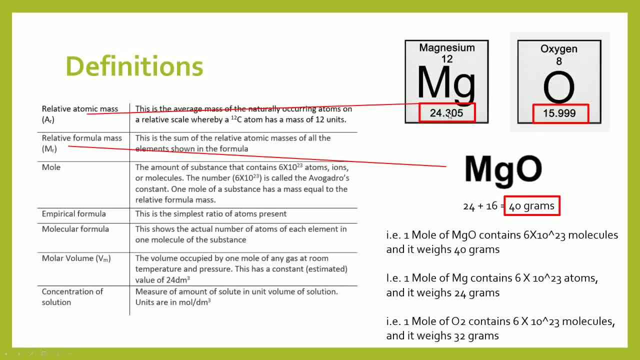 weight of a magnesium atom: okay, which is the relative atomic mass. Oxygen- okay, they're always in molecules- O2, will contain 6 times 10 to the power of 23 molecules. again, It'll weigh 32 grams, because the relative formula mass is 16 plus 16, which is 32.. So please get your head around this. 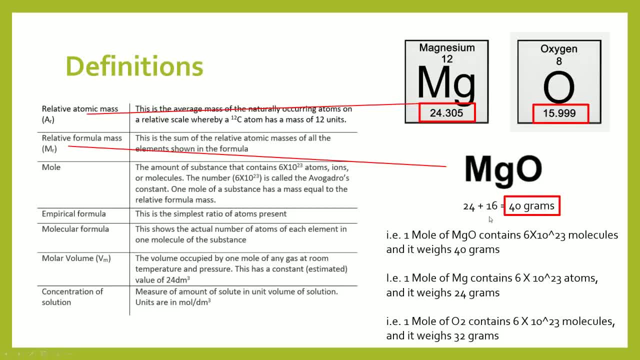 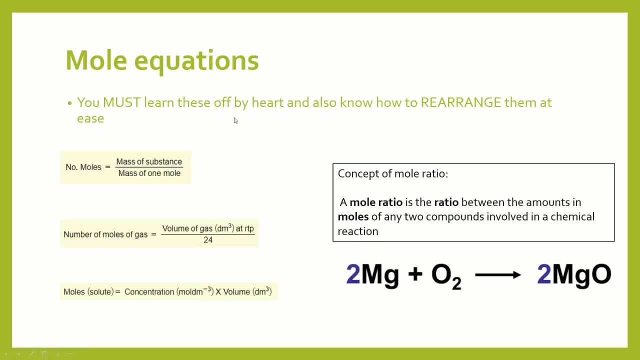 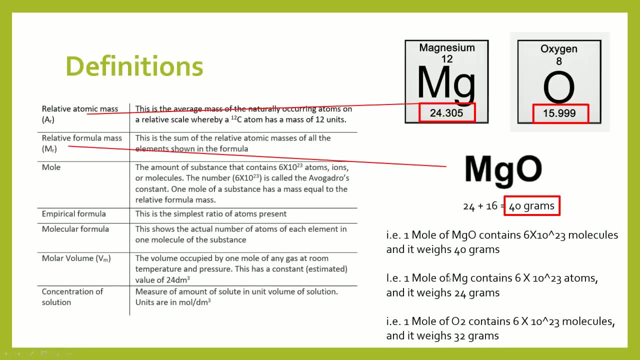 because this is extremely important. So when we start to look at mole calculations- right, so all the calculations that we'll be doing will be about moles, and this is the concept that we talked about before. okay, One mole will be the mass. well, one mole has the mass of the relative. 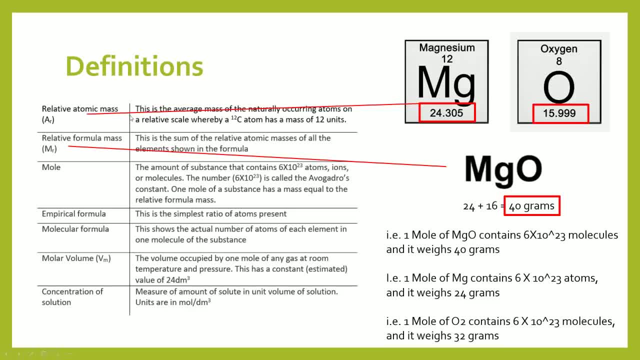 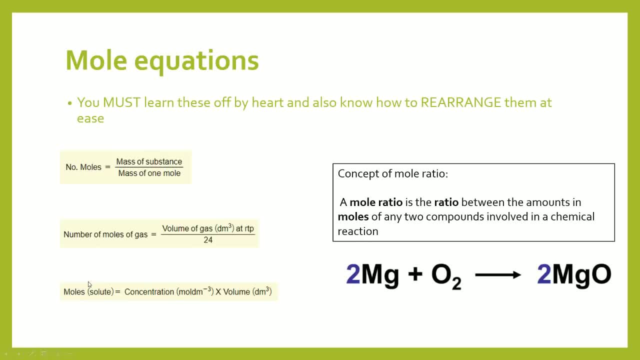 formula, mass or the relative atomic mass if there are just a single atom. okay, So there are three main equations that you need to know, and it's these three here, And you need to be able to memorize this and be able to rearrange them off by heart. You need to. 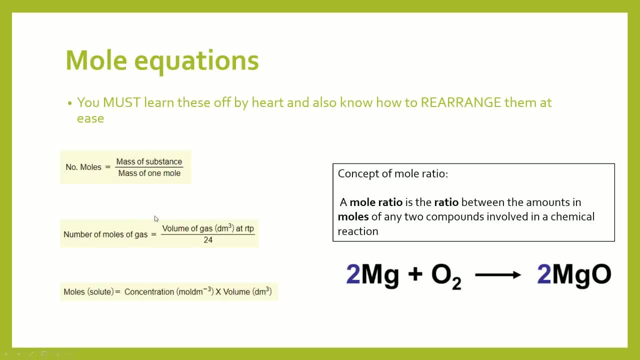 be very familiar with these three equations. Also, you do need to know the concept of mole ratios. We briefly touched on this before, but a mole ratio is the ratio between the amounts and moles of any two compounds involved in a chemical reaction. So you know, if just take a look at 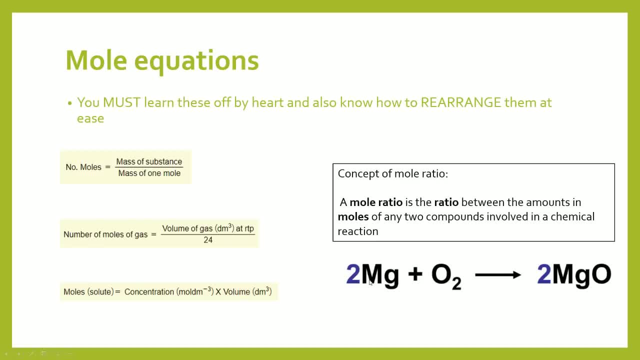 two separate you know substances here, For example magnesium and magnesium oxide. If one mole is used, then also one magnesium oxide mole will be formed in this particular equation, because the ratio between magnesium and magnesium oxide is one to one or two to two, which cancels. 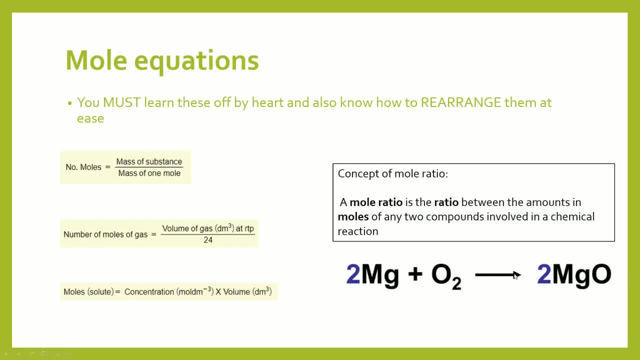 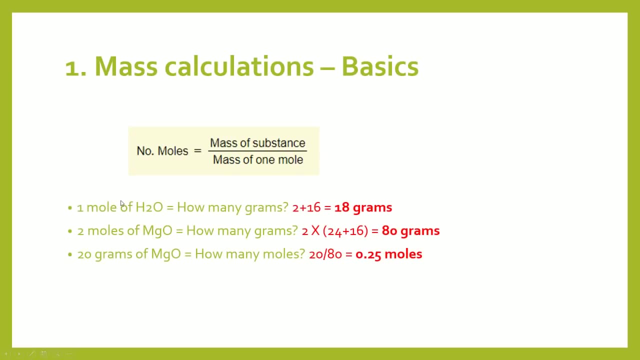 out to one to one, And you'll sort of understand this a bit more when we go through certain examples. but for now, please make sure that you understand these three formulas. So we're going to go through the use of each of these formulas one by one. So in terms of mass calculations, 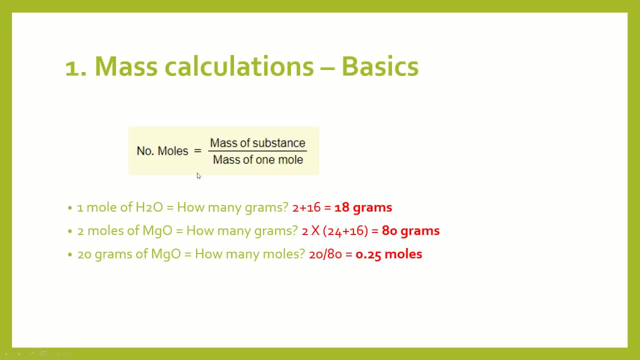 these are that you know. let's take a look at some examples using the basics here. So one mole of water which is H2O, how many grams is that going to be? You need to think to yourself. well, okay. 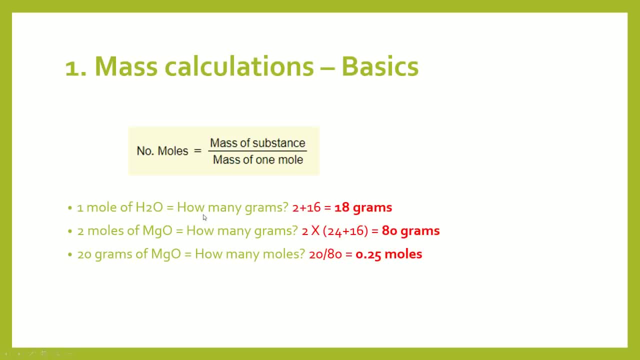 so we talked about one mole having the relative formula mass. So the relative formula mass of H2O is just the added atomic masses, which is 18, because you add two to 16.. Two moles of magnesium oxide, which is 18,, which is a relative formula mass, which is 24 plus 16,, which is 40. But you 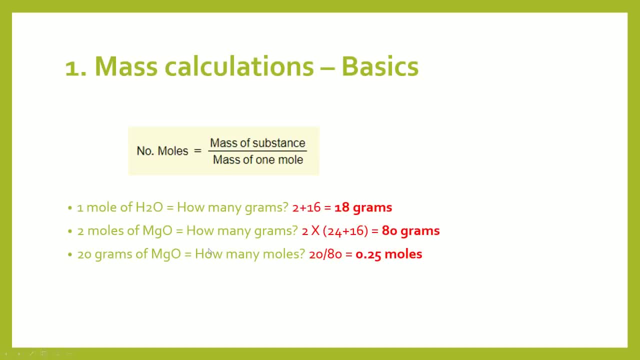 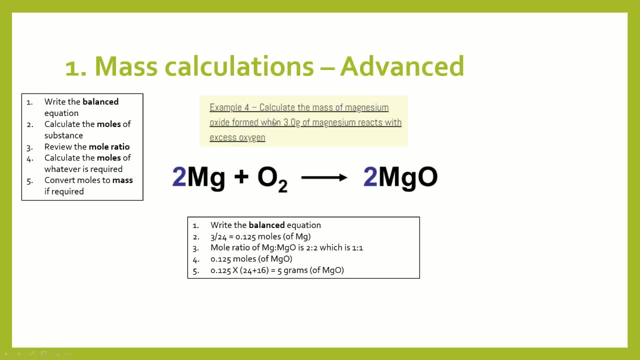 times that by two, because 40 is the mass of one mole. You've got two moles here, so that's 80 grams and you get the gist. So let's take a look at a bit more of a difficult example. So it says: 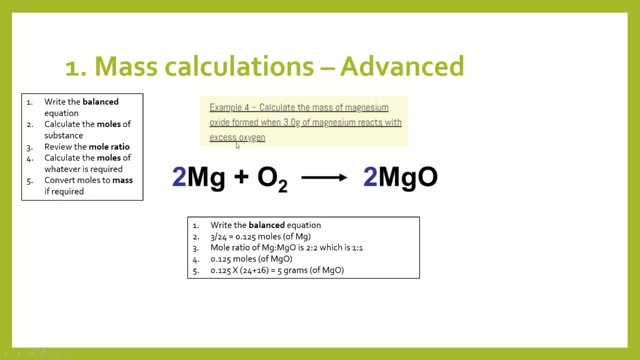 calculate the mass of magnesium oxide that is formed when three grams of magnesium reacts with excess oxygen. So I've wrote down a couple of steps here. First of all, you need to have a balanced record of all the moles of whatever substance that is in question In this equation we're talking. 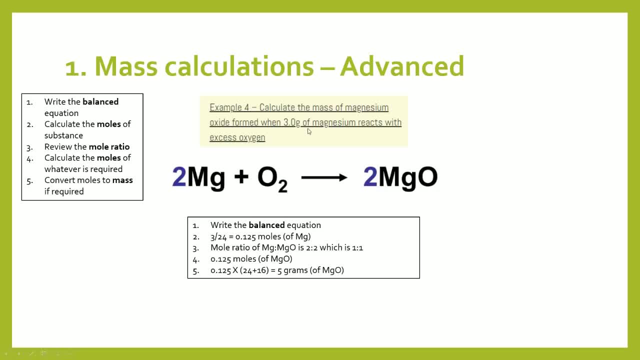 about magnesium. So they say three grams of magnesium. So you need to figure out well how many moles are three grams of magnesium. And then step three is to review what the mole ratio is, because they're asking for magnesium oxide. So then you take a look at the mole ratio between: 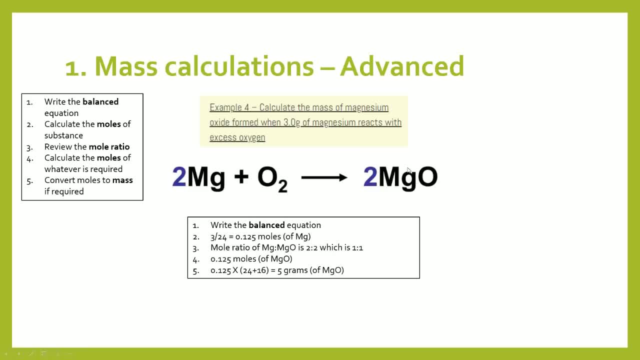 magnesium and magnesium oxide to calculate how many moles of magnesium oxide was formed from the ratio reaction. Once you know how many moles of magnesium oxide was formed, then you simply use the equation that we talked about before, this equation here to figure out what the final mass of the magnesium 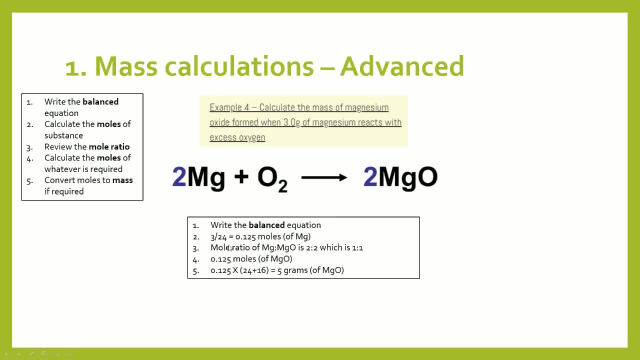 oxide was So, therefore, let's go through those steps one by one. You've got the balance equation, and so, if you want to calculate the moles of magnesium, all you need to do is chuck it into the formula, and the equation becomes three grams divided by the relative formula: mass of magnesium. 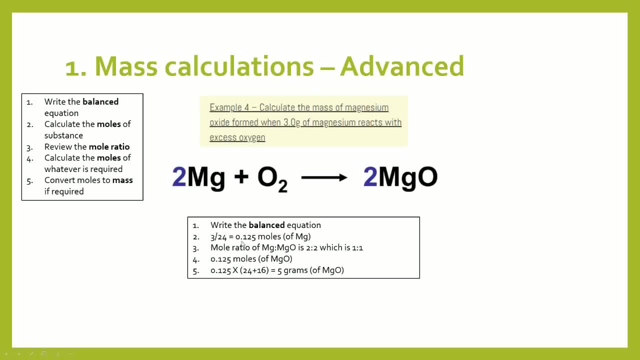 which is 24.. So you get 0.125 moles of magnesium. that was used in the reaction. So if 0.125 moles of magnesium was used, then you'd figure out the mole ratio right. So you've got the number two. 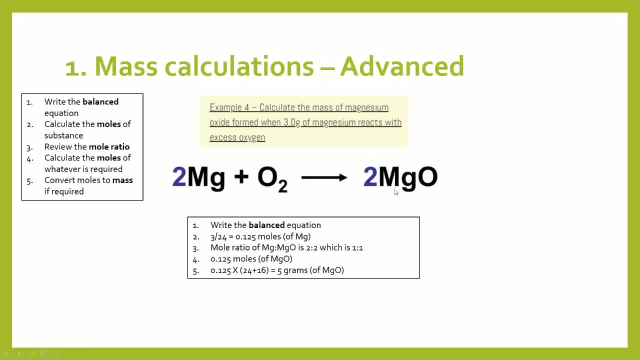 in front of magnesium and you've also got the number two in front of magnesium oxide, giving you a ratio of directly. What that means is, since 0.125 moles of magnesium was used, 0.125 moles of magnesium oxide has been formed. 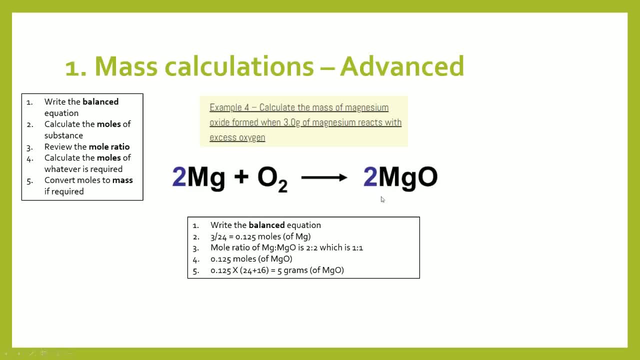 Now that you know that 0.125 moles of magnesium oxide has been formed, you basically re-chuck it back into this formula. you rearrange everything and you get 0.125 times the relative formula mass, And that gives you 5 grams, which is the mass of magnesium oxide that was formed. 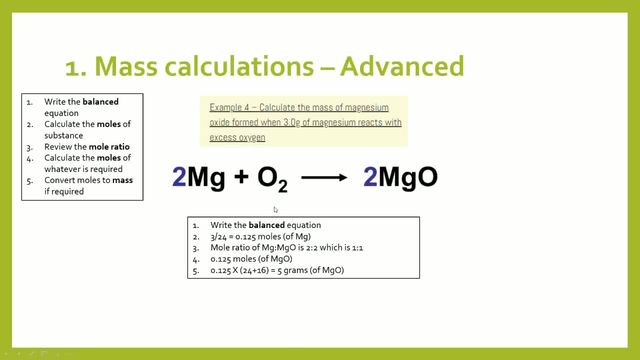 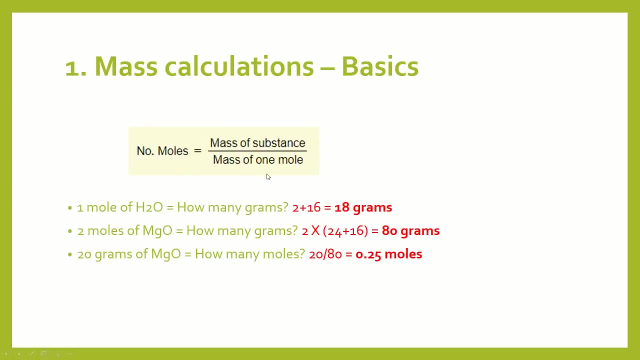 So the main key point here, guys, is to initially calculate the moles and take a look at the mole ratio, take a look at the moles of whatever substance that was formed, and then convert that back into mass, And that's all done using this simple formula, as we took a look at before. 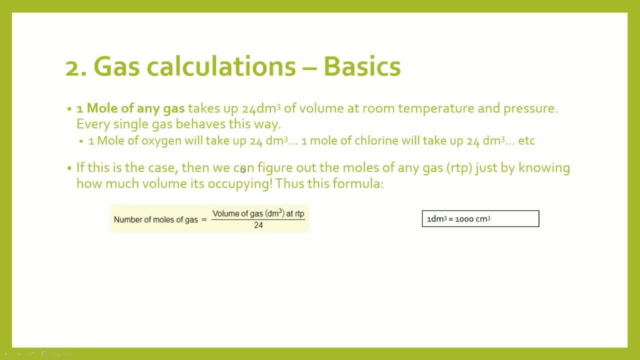 So second of all is gas calculations, The basics of gas calculations. is there's a really important idea here that 1 mole of any gas- right, it doesn't any gas- will take up 24 decimeters cubed of volume at room temperature and pressure? 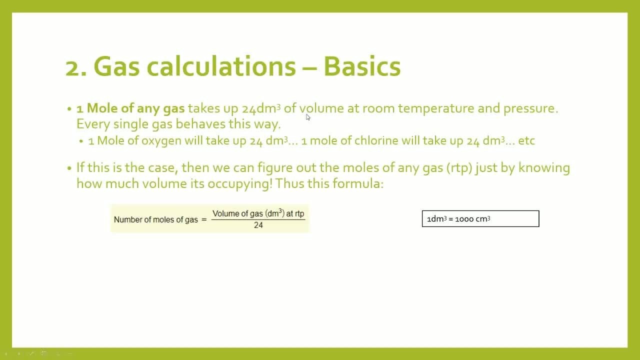 Okay, so every single gas behaves this way. so that means 1 mole of oxygen will take up 24 decimeters cubed. 1 mole of chlorine gas will take up 24 decimeters cubed. every single gas will take up 24 decimeters cubed. 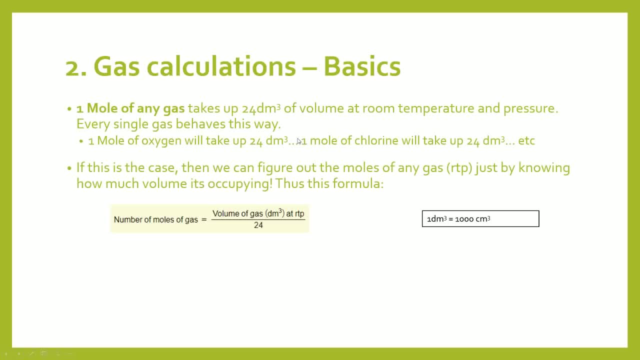 Okay, 1 mole of that particular gas. that is Okay. so if that was the case, then we can actually figure out the moles of any gas just by knowing how much volume it's occupying, and vice versa. So therefore, we have derived this formula whereby the moles of any you know particular gas, at room temperature and pressure of course, is the volume of the gas divided by 24, because 24 is how much 1 mole would occupy. 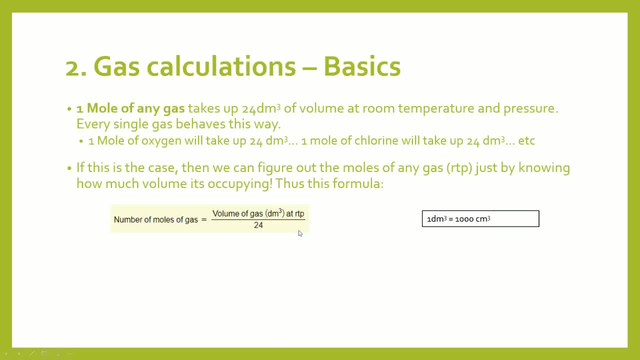 Remember, decimeters cubed is 1000 centimeters Centimeters cubed, then quite often they will tell you they may say that the volume is, you know whatever, in centimeters cubed. so you always have to divide it. or you know you always have to convert it back to decimeters cubed before applying this equation. 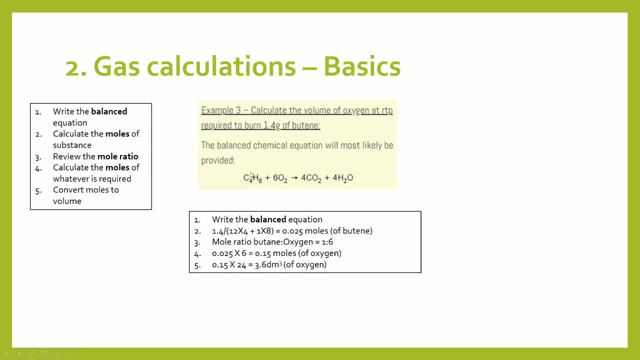 So let's take a look at an example. It's actually very similar to what we took a look at before. So the example says: calculate the volume of oxygen at room temperature and pressure required to burn 1.4 grams of butane. 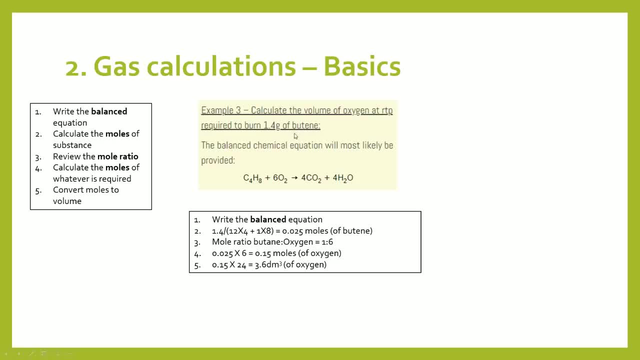 Great. So 1.4 grams of butane? We take a look at the balance equation here and we think: well, 1.4 grams of butane, how many moles is that? We always want to think about the moles, not the mass right. 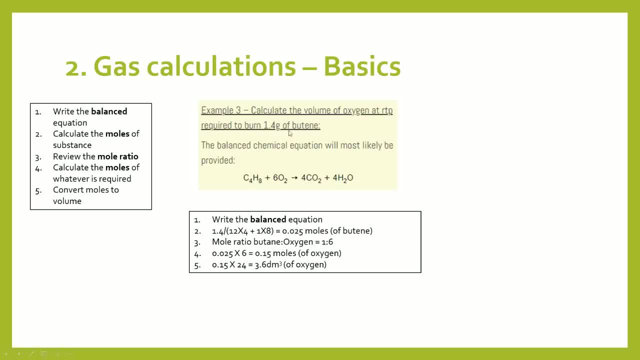 So 1.4 divided by the relative formula, mass of butane, which is, I suppose, 12 times 4 from the carbons and 1 times 8 from the hydrogens, giving you 0.025 moles of butane that was used in the chemical reaction. 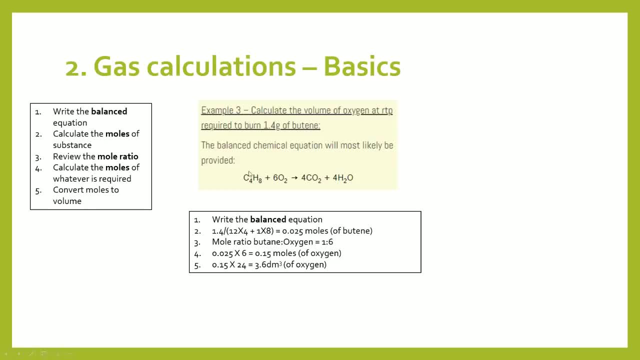 The mole ratio here is 1 to 6.. For every mole of butane you get 6 moles, So 0.025 moles of oxygen being used. What that means is if 0.025 moles of butane were used, then 6 times that would have been used in terms of oxygen. 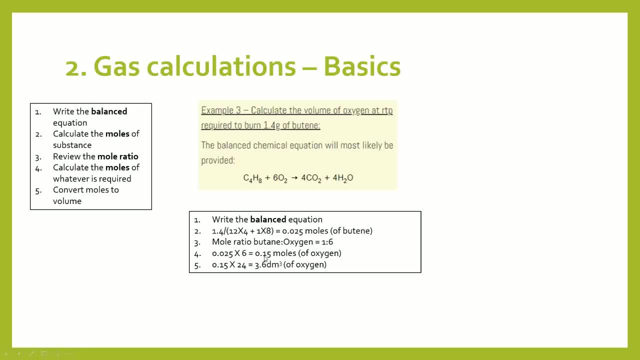 So you simply times 0.025 by 6, and you get 0.15 moles of oxygen. Now that you have the moles of oxygen, you can actually calculate the volume using the equation before. So 0.15 times 24.. 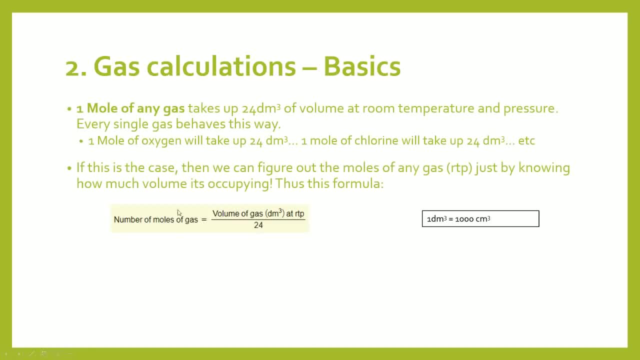 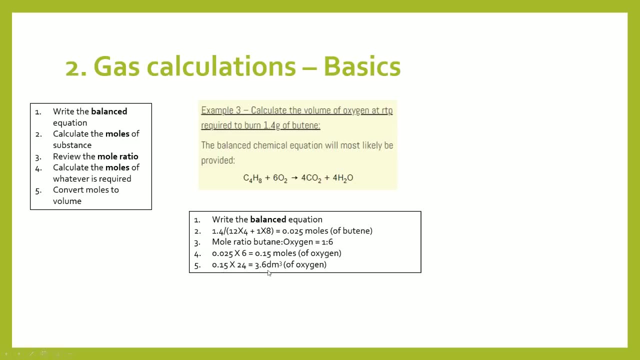 Okay, so this is a rearranged form of the equation, obviously, because now you want volume. So volume is moles times 24.. So the moles of 0.15, you times that by 24, you get 3.6 decimeters cubed of oxygen. 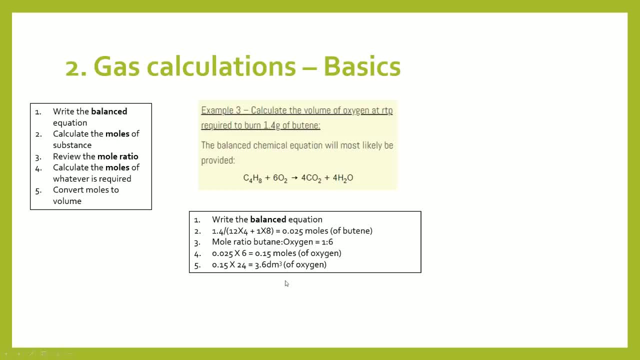 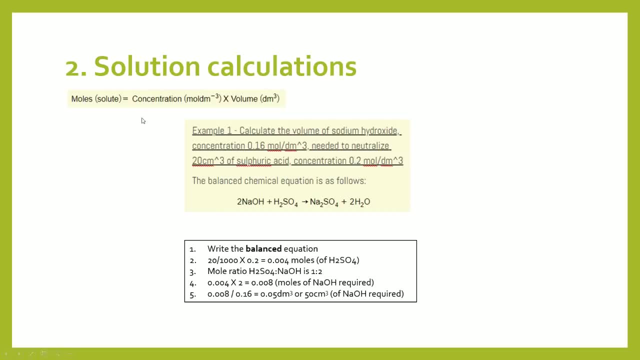 That is the volume of oxygen that is required to burn 1.4 grams, okay, of butane. The third one is solution calculations whereby the- you know the formula- is moles of the solid, or you know whatever it is, is the concentration times volume. 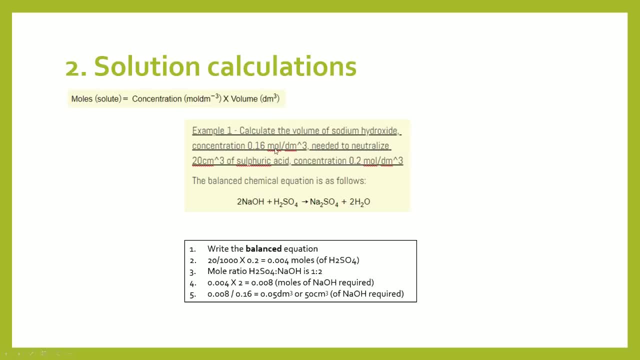 Take a look at this example here. Calculate the volume of sodium hydroxide. So this is the volume of sodium hydroxide concentration of 0.16, needed to neutralize sulfuric acid, which has 20 centimeters cubed and 0.2 moles per decimeters cubed. 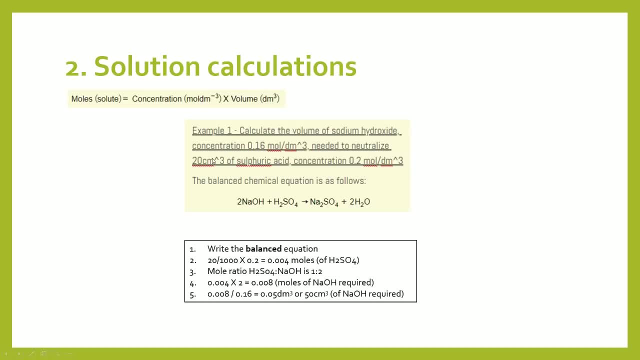 So, of course, this is the concentration, This is the volume of sulfuric acid. So initially, immediately, you can see that you can calculate the moles of sulfuric acid. Okay, so what is the moles of sulfuric acid then? 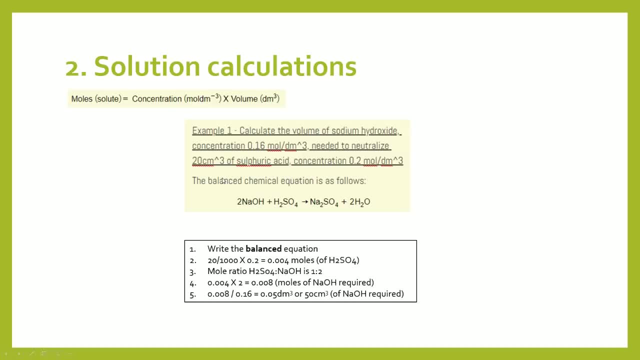 Okay. so you apply this equation Here and you get concentration times volume. So 20 divided by 1,000, because this is in centimeters cubed. You want to convert that to decimeters cubed- 20 divided by 1,000,. you times that by 0.2, which is the concentration, and you get 0.004 moles of hydrochloric- sorry, hydrogen sulfate.